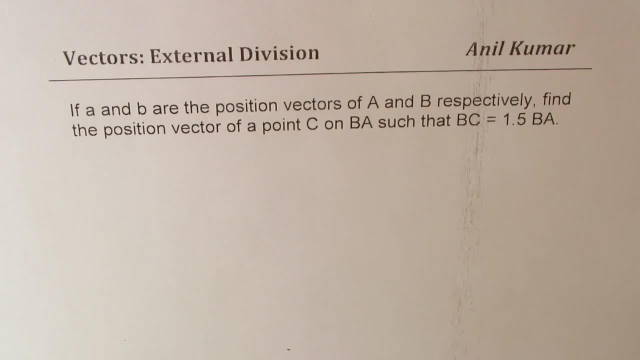 I'm Anil Kumar sharing with you a very important test question on external division of segment using vectors. If a and b are position vectors of a and b respectively, find the position vector of a point c on b a such that b c equals to 1.5 b a right. So let's make a small diagram here. 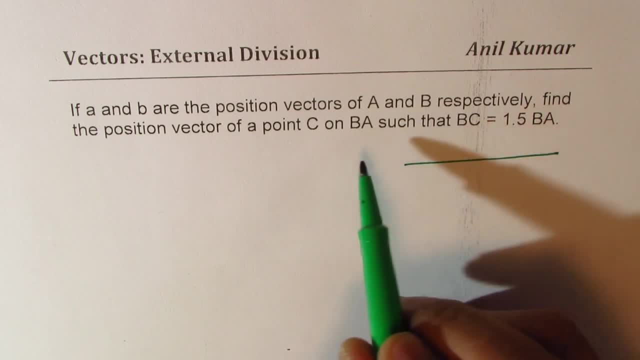 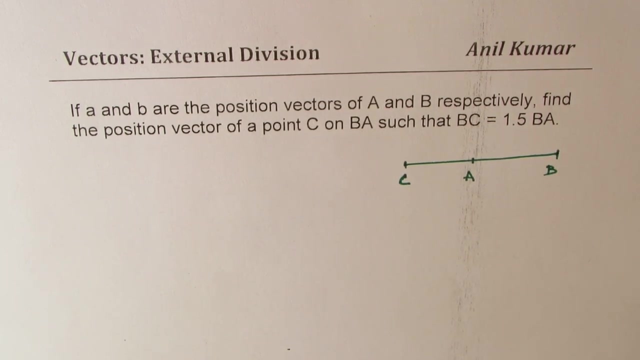 So what we have here is we have a to b and a point c. here We are given that b c is equals to 1.5 times b a. That means this side is 1.5 times b a. So what we have here is that b c is equal to. 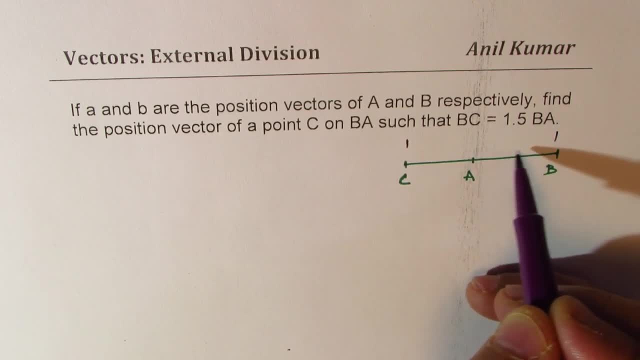 1.5 times b a. So what we have here is that b- c is equal to 1.5 times b? a. So let's make a small diagram: 1.5 times BA, right? So if this is x, in that case B to C is 1.5x. That is what we. 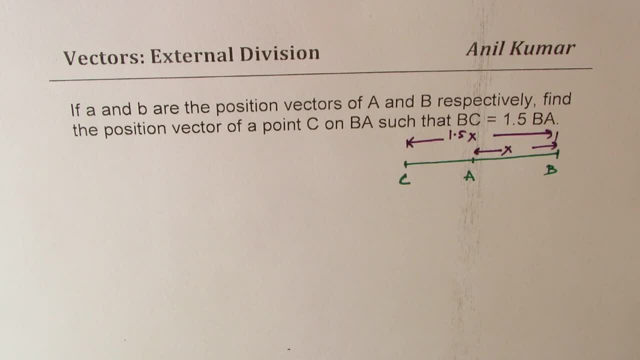 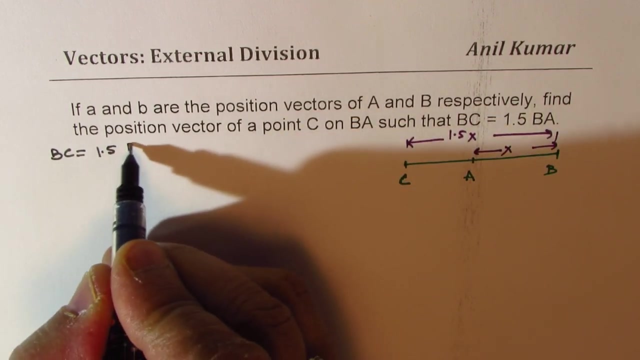 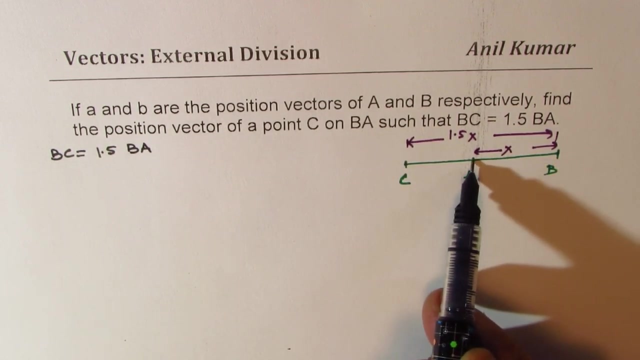 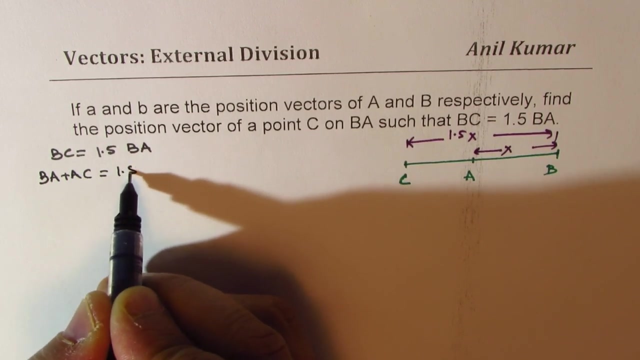 are given right Now. let's try to understand this. So in this particular case, we are given that B to C is 1.5 times BA. So we could write B to C as combination of BA and AC, right? So B to C could be written as BA plus AC, which is 1.5 times BA. So now, 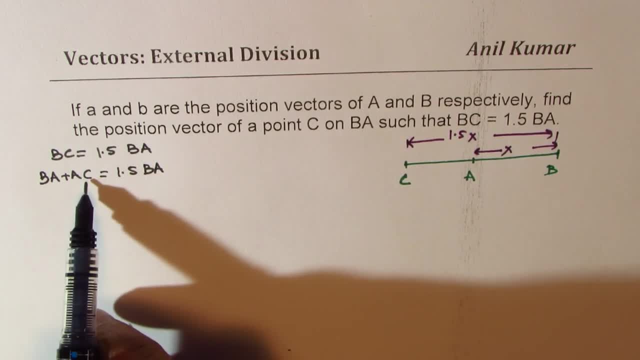 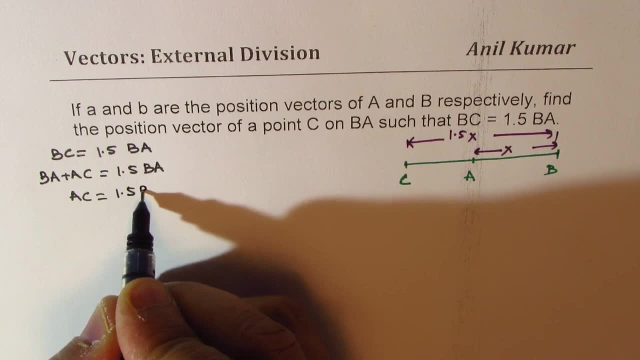 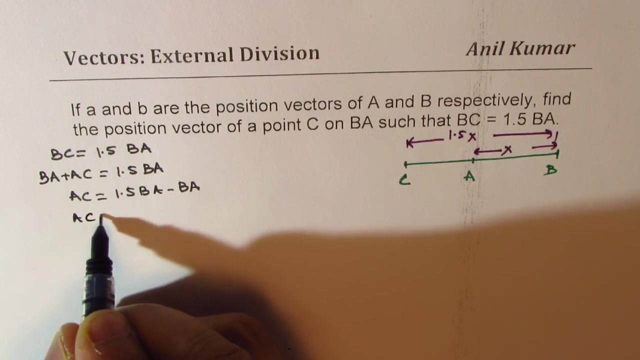 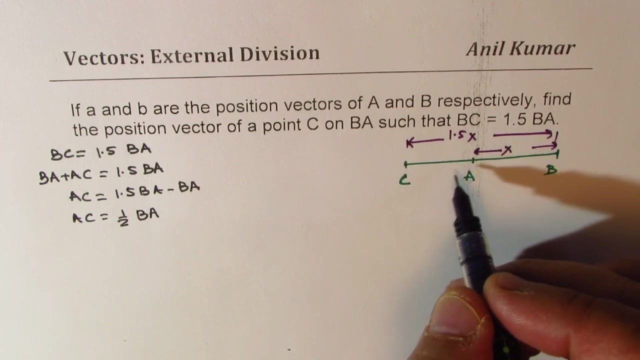 we could write what AC is right. So AC will be 1.5 times BA minus BA, correct? So which is: which means that AC is half of BA. So that means that AC is half of BA. So that means that AC is. 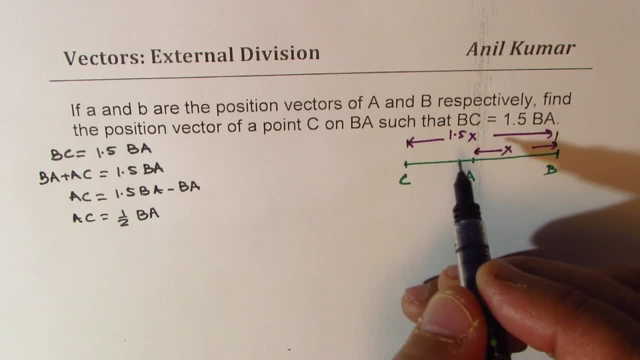 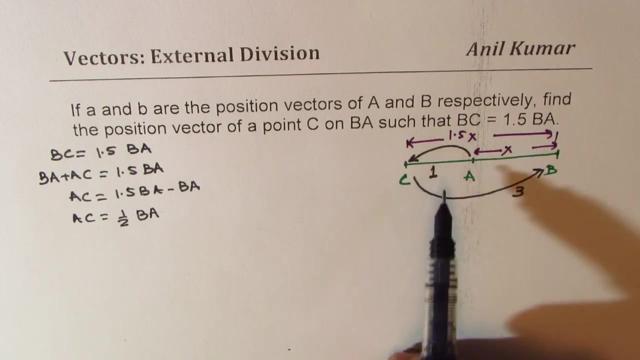 there could be three equal divisions, right? So it could be written as from A to C: if the distance is one unit, then from C to B it will be three units. So you could also see that point C is externally dividing AB in the ratio of 1 is to minus 3.. So from here you could conclude that 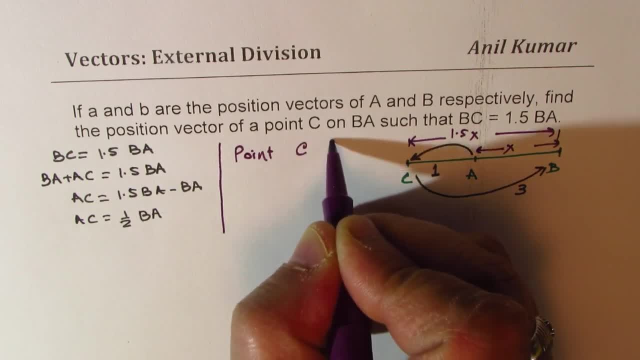 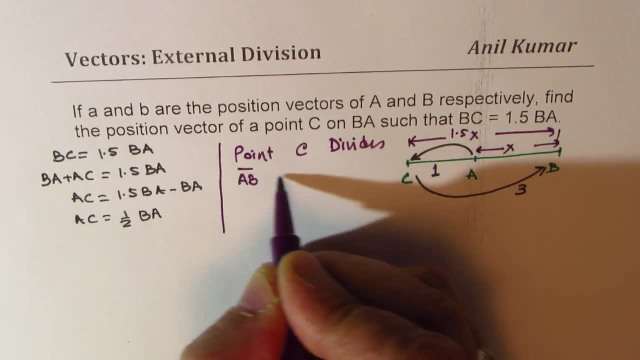 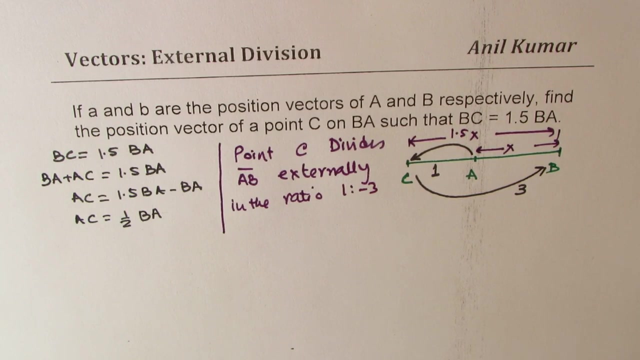 point C divides AB externally, right in the ratio of 1 is to minus 3, correct? So, since C is on this side, right? so A to C. if you are taking this side as positive, then going to the other way will be considered as negative. So that is how. 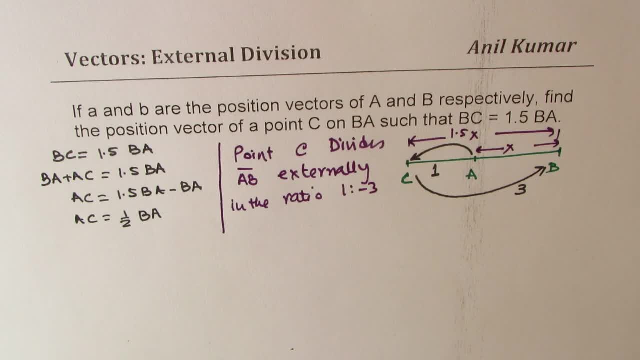 we could see as if it is an external division. Now you can use the section formulas for external division to find the coordinates of point C right. So from here you could see that the coordinates for point C is 1 times B right, Or 1 times B. 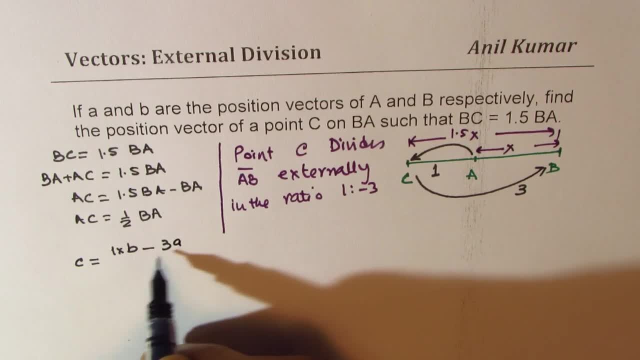 minus 3 times A over 1 minus 3, correct. So that is how you get the coordinates of point C, which is equal to B minus 3A over minus 2, correct? or you could write this as 3a minus b over 2.. 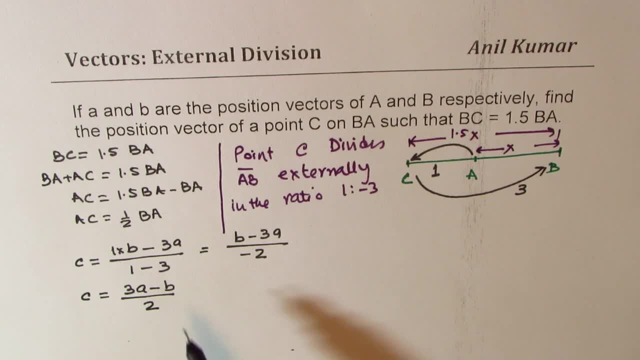 So I hope the steps are clear. So this in this particular case: we first showed that c is dividing ab externally in the ratio of one is to three, And then we used our section formula to find the result that c should be equal to half of 3a minus b. 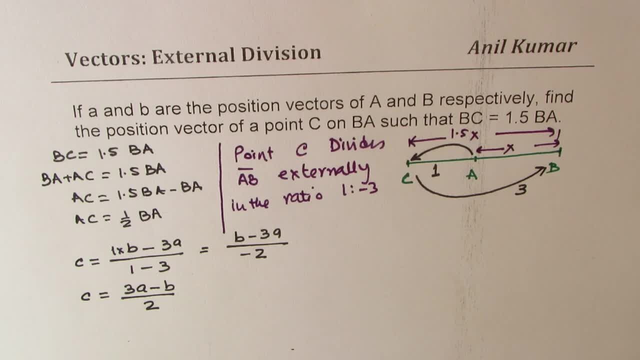 Okay, So that is how you could easily do this question. I'll provide you with a link on working with the section formula as such, So we'll derive this particular equation right Using section formula and then we'll use it, Okay.